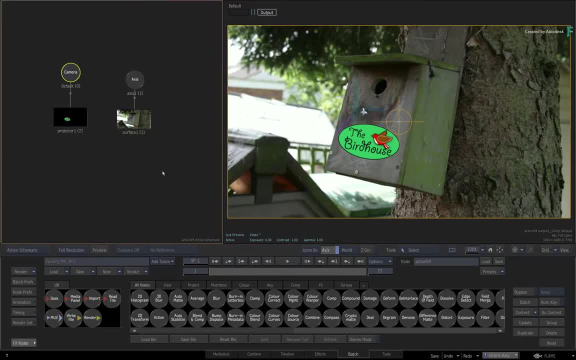 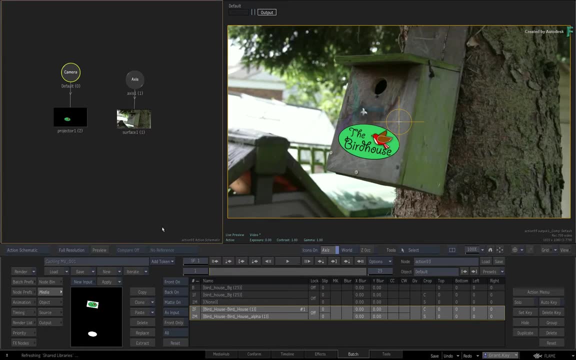 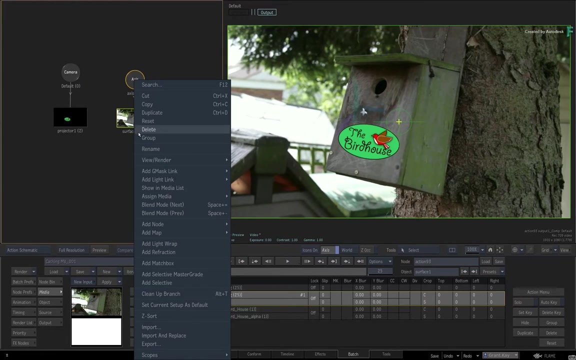 Now there are plenty of techniques to do this, but I'll apply the Motion Vectors to the surface and use a projector to perform the motion warp tracking. So select the background in the Media List and Action Schematic. Apply a Motion Vectors map with either the context menu or the Action node bin. 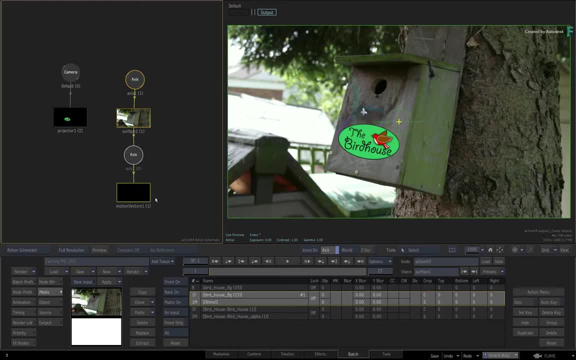 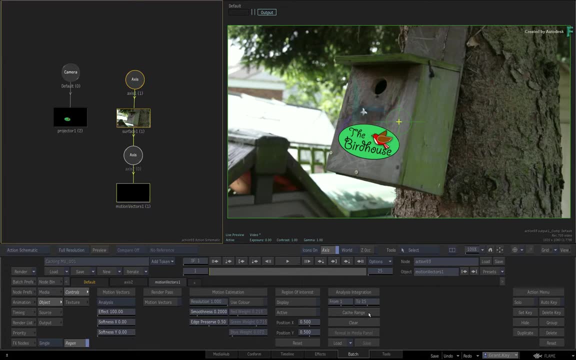 Now to create a proper Motion Vectors cache with the required integration calculation, you must click the CACHE RANGE button in the Motion Vectors panel. You can also use the Motion Vectors Map menu. The Analysis Integration Frame Range should match the duration of Batch to work correctly. 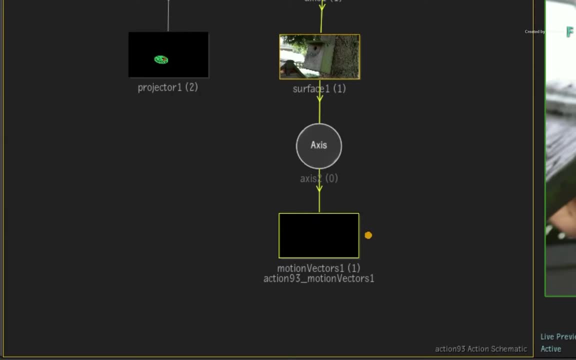 Now a few things happen at this point. Firstly, you get an orange dot next to the Motion Vectors map which tells you it's using a cached clip. Secondly, the name of the cached clip is listed under the map's name. The standard formatting is the same as before. 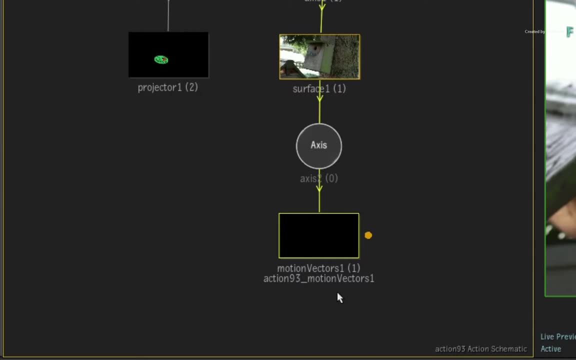 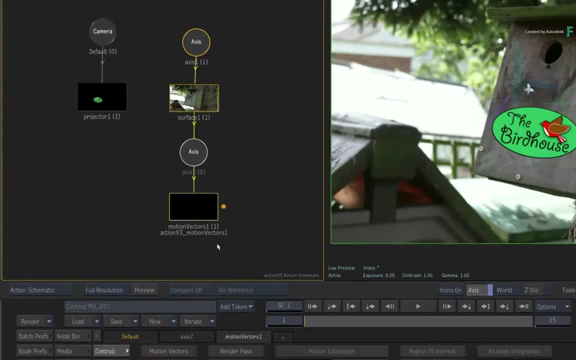 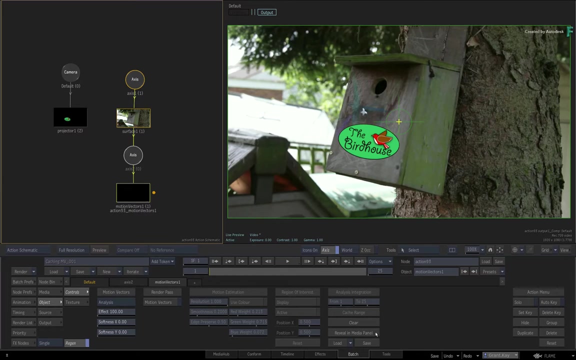 The name of the parent node is the same as the name of the Motion Vectors map. Finally, if you want to see the cached Motion Vectors clip, you could reveal it through the context menu or button in the Motion Vectors menu. You can also double-click on the orange dot and it will reveal itself in the Media Panel. 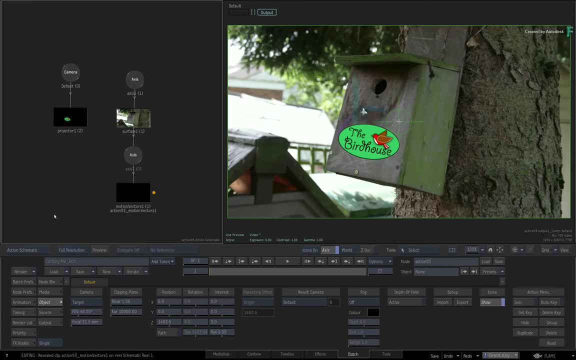 Now. you'll come back to the cached clip very shortly, but to complete this example, go to the Projectors Tracking menu and add a Reference Frame to lock the logo to the track. You should see the tracked result as you scrub the time-bar. 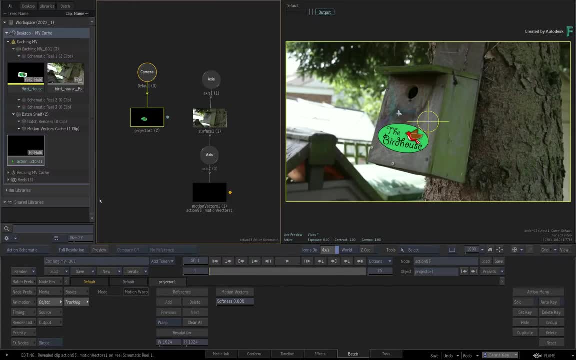 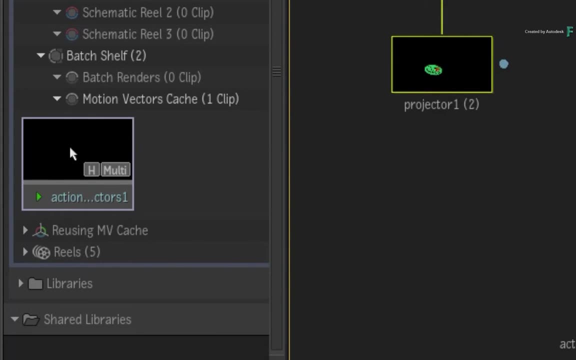 Now, the cached Motion Vectors clip contains the Motion Vectors, as expected, but it also contains all the integration data used for Motion Warp Tracking and 3D Tracking. Therefore, the cached clip's only use is within Action Image and the Gmask Tracer. 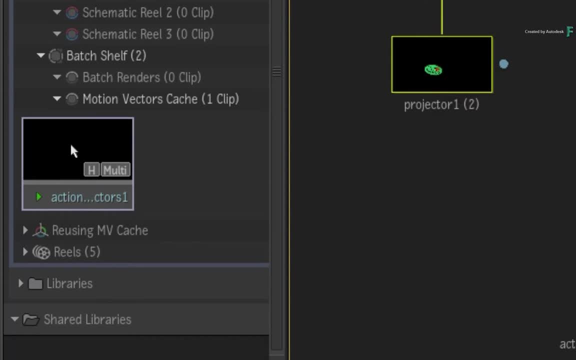 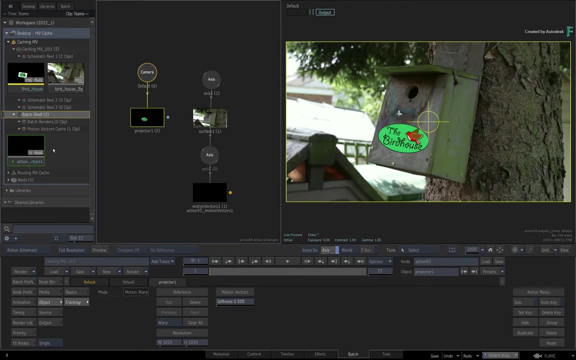 This is the reason why it's stored in a Batch Shelf and not in the Batch Schematic Reels. Schematic Reels contain clips that you use as part of the node flow graph, And Batch Shelves contain any final renders and now cached Motion Vector clips. 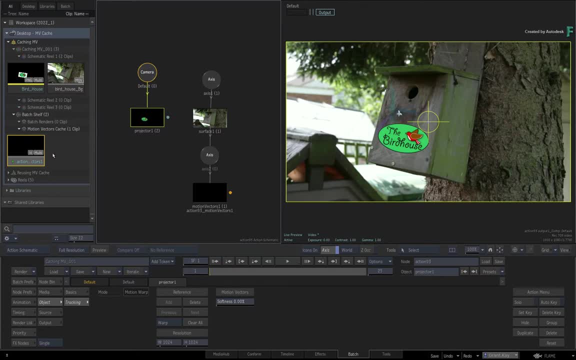 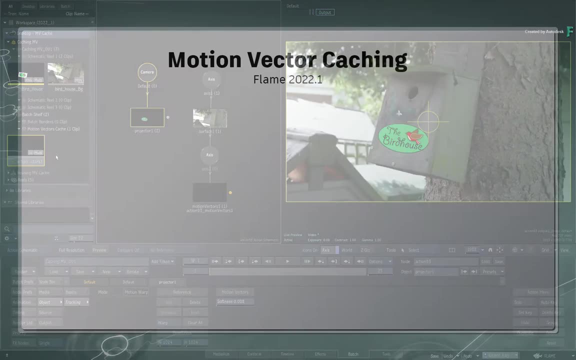 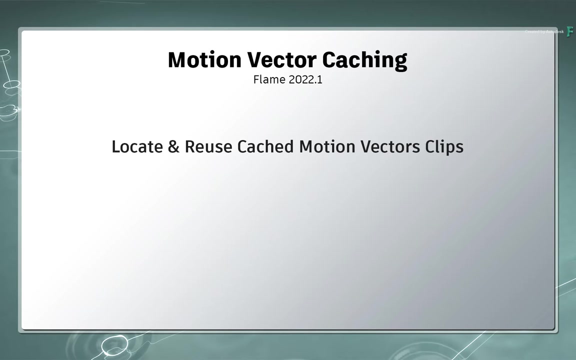 that you don't need in the current flow graph, but are considered as part of the Batch Group. This design benefits you in a few ways. Firstly, you know where your Motion Vector Cache is… And it can be used multiple times within the same Batch composite. 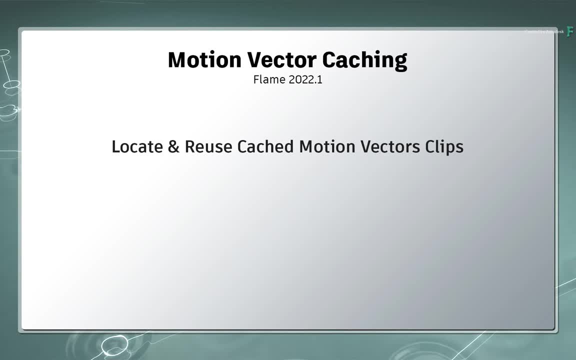 No need to re-cache every time. Secondly, the Motion Vectors Cache is an actual clip in the Flame Database. Therefore, you can reuse it in other Batch Groups or BFX And finally, being a cached clip, it can be wired to other machines…. 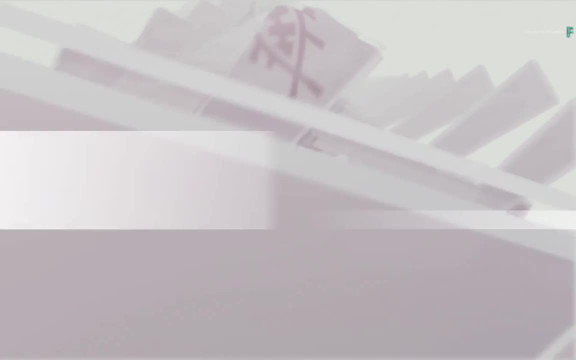 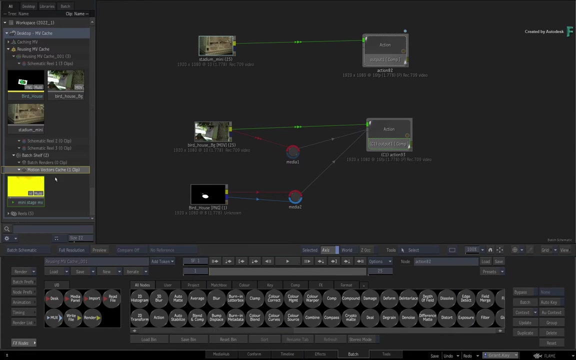 as well as backed up as part of an Archive. So in creating the Motion Vectors Cache… It appears in a Batch Shelf called Motion Vectors Cache… And it does not appear in the Batch Schematic by default To reuse this cached data…. 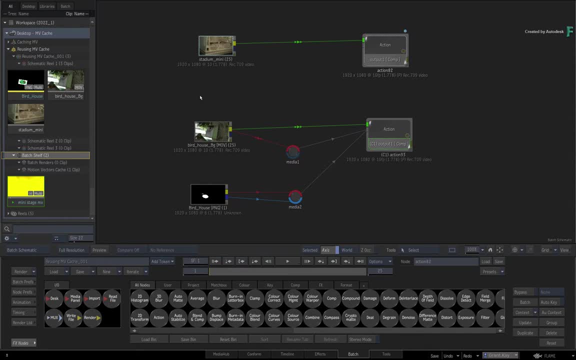 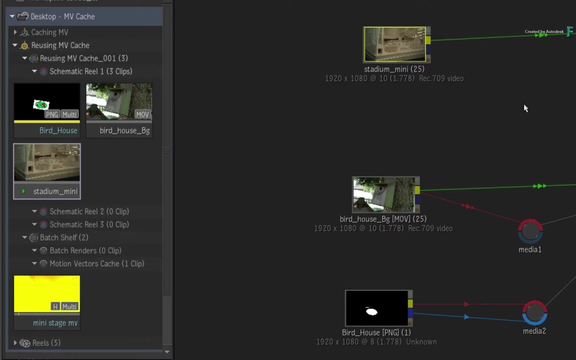 The recommended workflow is to load it directly into the Motion Vectors Map… In either Action Image or the Gmask Tracer. Now in this Batch Group… You already have a cached Motion Vectors clip that was created earlier… And it belongs to this shot that you would like to 3D track. 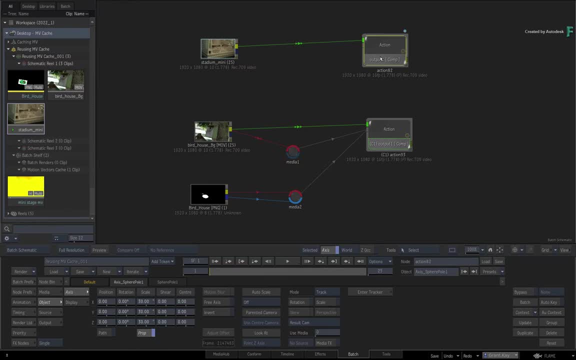 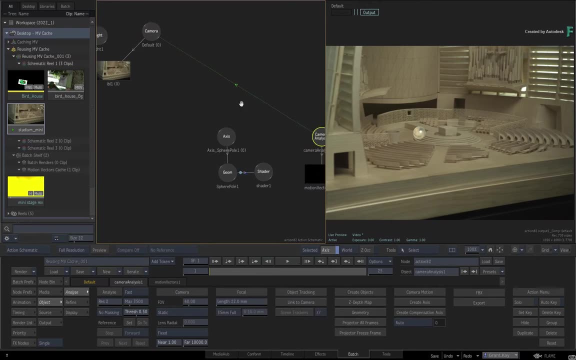 So, to reuse a Motion Vectors Cache… You go into the Action node… And since this is a 3D tracking example… You add a Camera Analysis to the 3D camera. This automatically adds the Motion Vectors Map… And you can look at its menus. 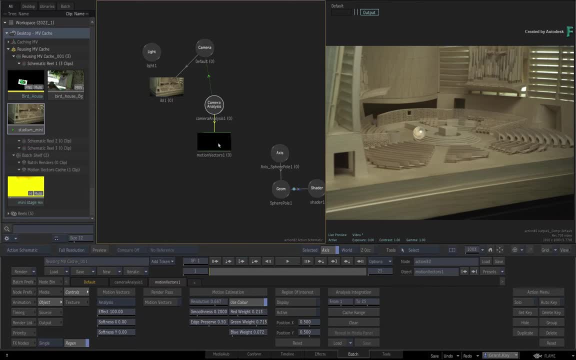 Now, there are many ways…. You can load a cached Motion Vectors clip. You have the contextual menus… The button in the menu… Or you can simply drag and drop the clip from the Media Panel. The cached indicator appears… And that's all you have to do. 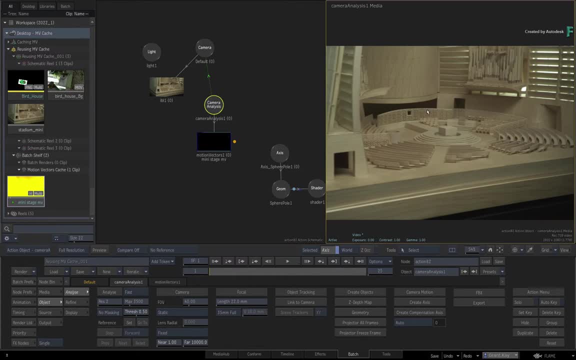 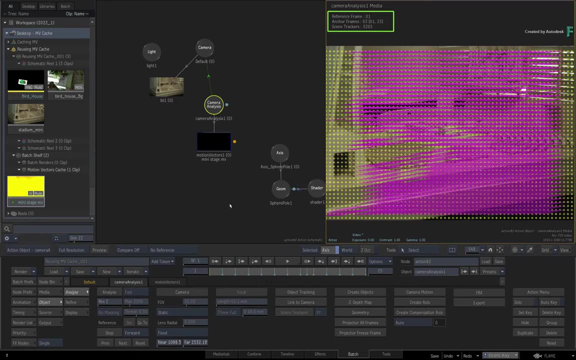 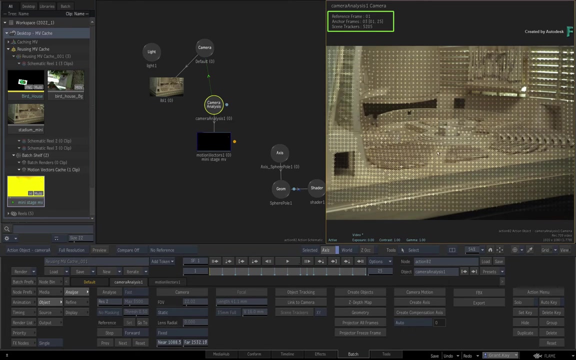 To quickly finish the 3D track… You go into Camera Analysis… And look at the Camera Analysis Media View… And analyse the shot. This should be incredibly fast. using the Cache Motion Vectors Clip. You'd now choose your points… Create a Scene Tracker Axis…. 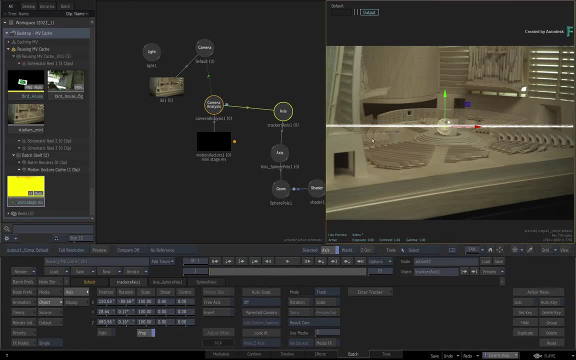 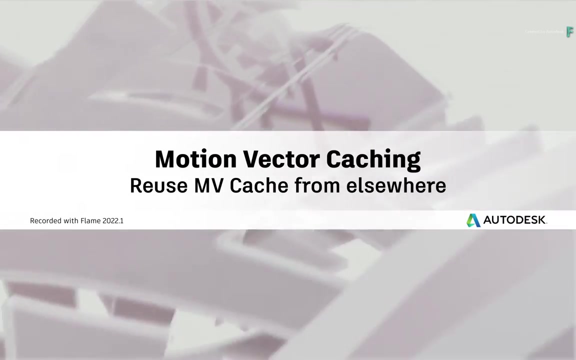 And integrate your objects into the 3D track composite. So this is using a cached Motion Vectors Clip…. That is already in the current Batch Group, But what if it was coming from somewhere else? Let's look at another example of loading a Motion Vectors Cache…. 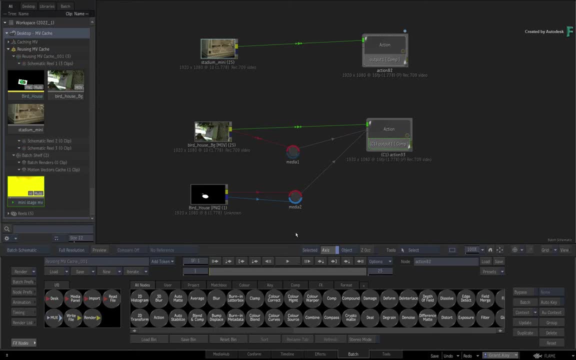 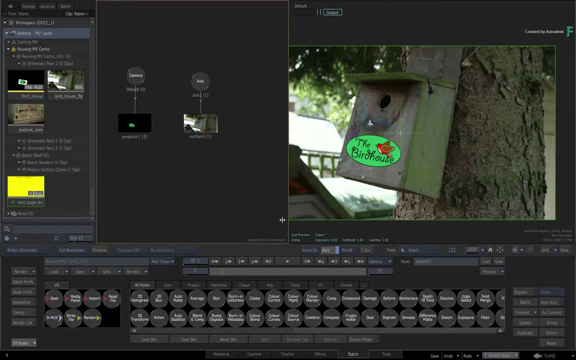 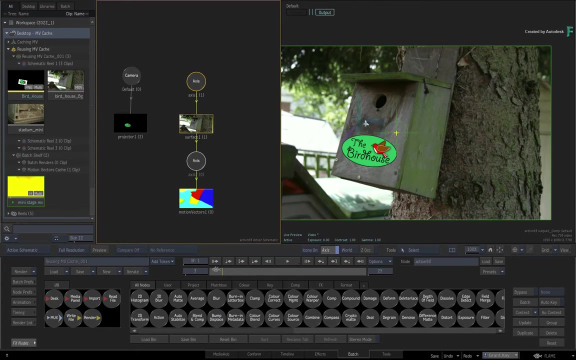 from outside the current Batch Group. Here you have the first composite without the Motion Vectors Map. So to perform the Motion Warp Tracking…. You add a Motion Vectors Map to the surface. object: To load a Motion Vectors Cache from outside of the current Batch Group…. 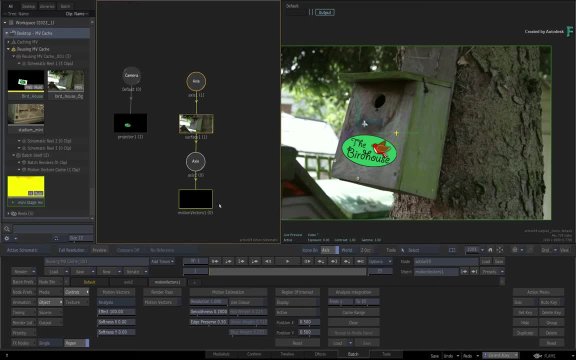 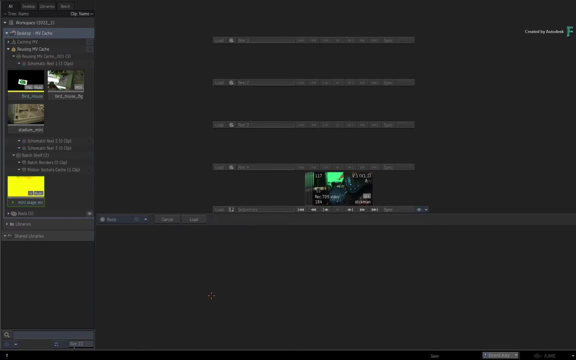 You can use the same operations as before: Drag and drop, contextual menu… Or click the LOAD button. Using the LOAD function… Will display the Media Panel and Reels view… And you can move around the workspace to find your cached Motion Vectors. 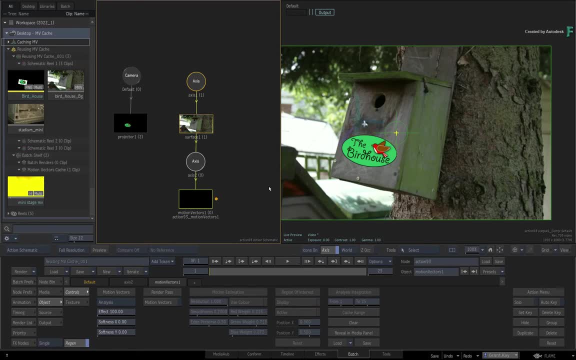 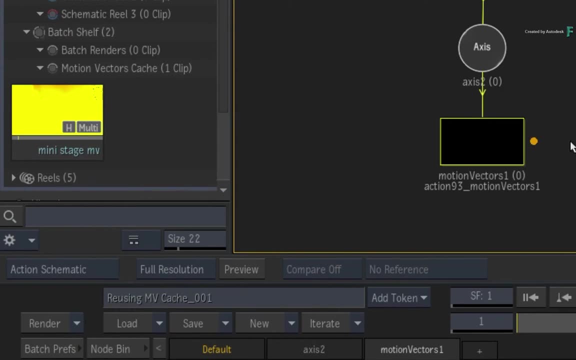 You'll use the cached Motion Vectors from the other Batch Group… But it could have been copied or restored from somewhere else. There is the cached status… And the name of the cached Motion Vectors is under the map. However, in this scenario…. 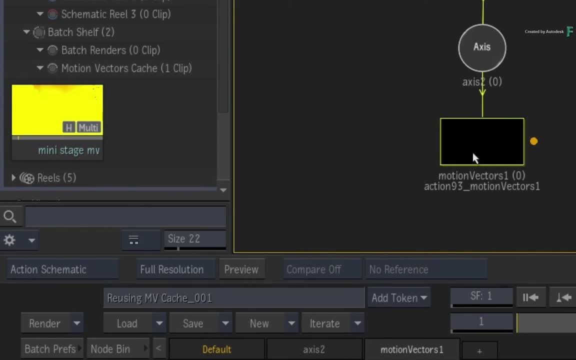 The Cached Motion Vectors Clip… Is being referenced to another Batch Group. Looking at the Batch Shelf… You only see the Motion Vectors Cache of the 3D tracked shot. So to ensure the Motion Vectors Cache is within your Batch Group…. 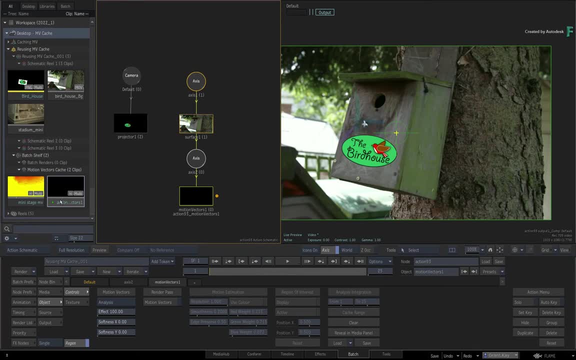 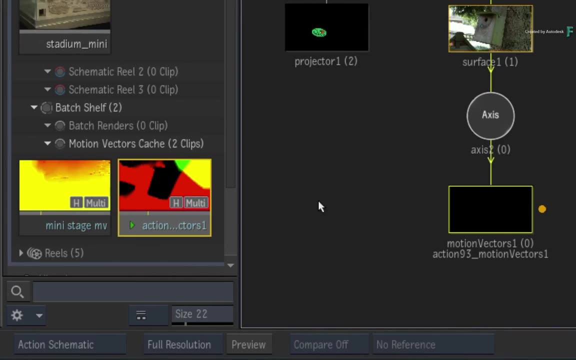 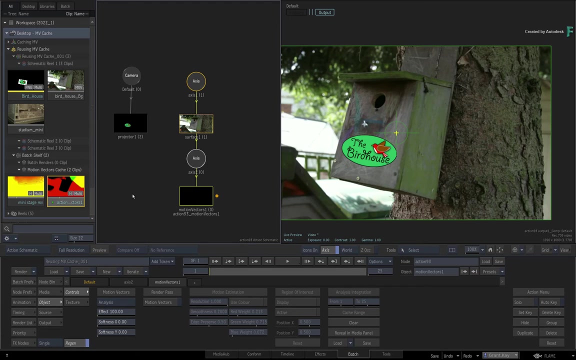 Click the SAVE button… And a copy of the Motion Vectors Cache will be created and contained within your current Batch Group. This ensures you keep everything together. Finally, it is very important to mention… That if you load a cached Motion Vectors Clip…. 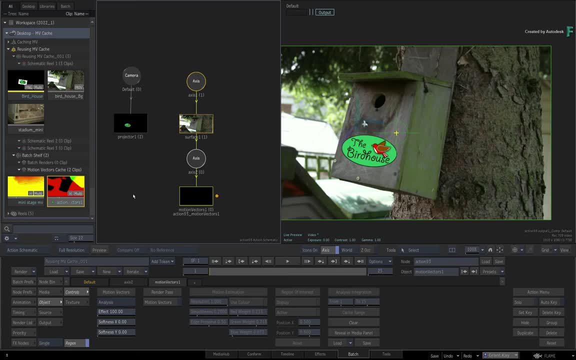 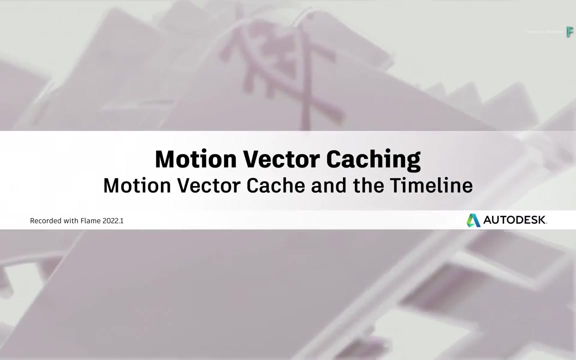 With a different start frame or duration… Flame will warn you of potential issues… And make the appropriate suggestions to work with that cache. And in some cases… You might need to recreate the Motion Vectors Cache for that shot. Now the workflow of using Motion Vectors Cache in the sequence…: 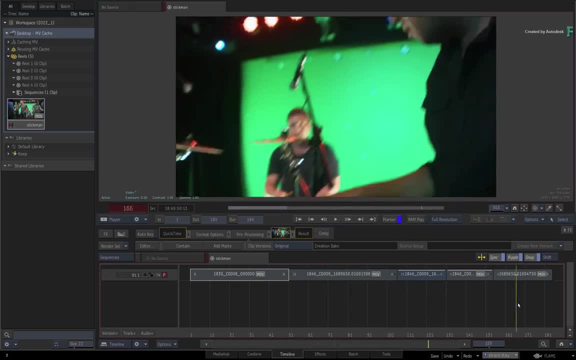 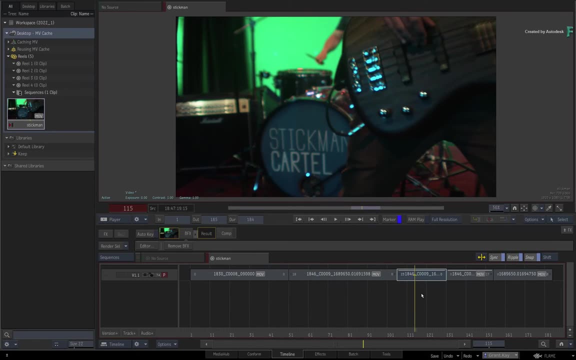 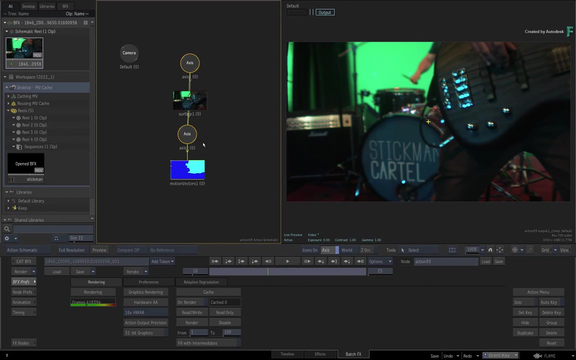 Is the same as working in Batch. The only key difference… Is that you don't have the Batch Shelf Reels to store the cached clips, So the saving is slightly different. For example… If you go into a BatchFX… And are working with a Motion Vectors Map….